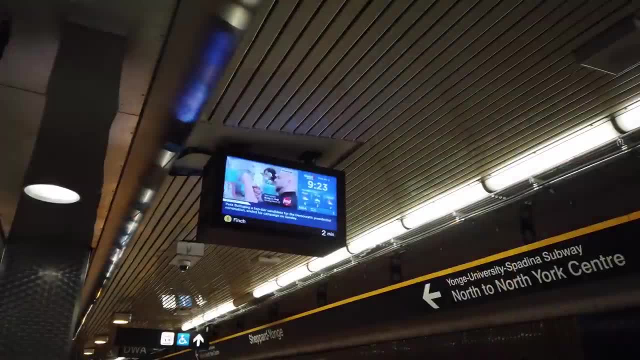 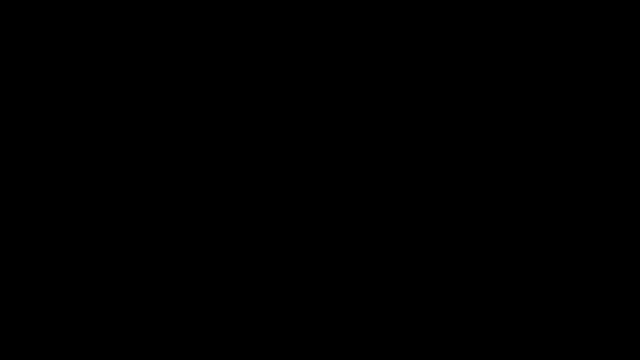 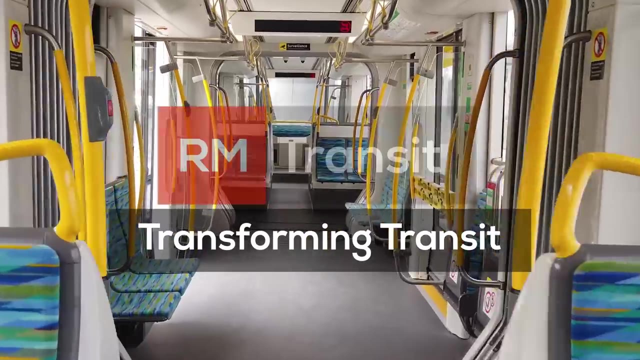 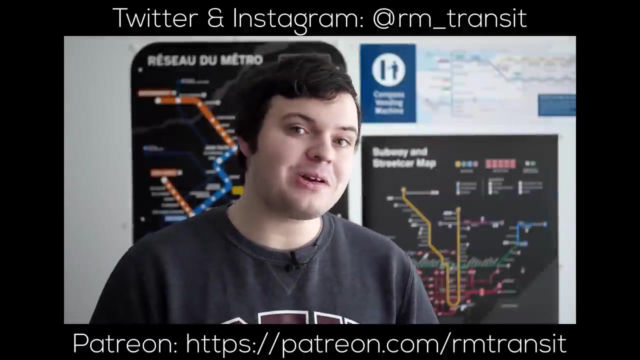 something else. Today we are really going back to basics. We're talking about why frequency is fundamental to good transit and how that's so often forgotten. Let's dive in. If you're watching this, chances are you may not be subscribed, So seriously consider doing it. 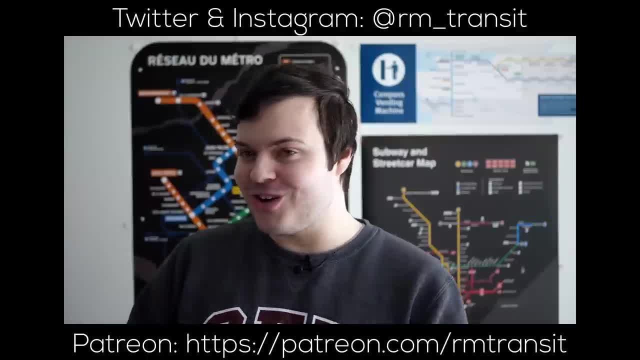 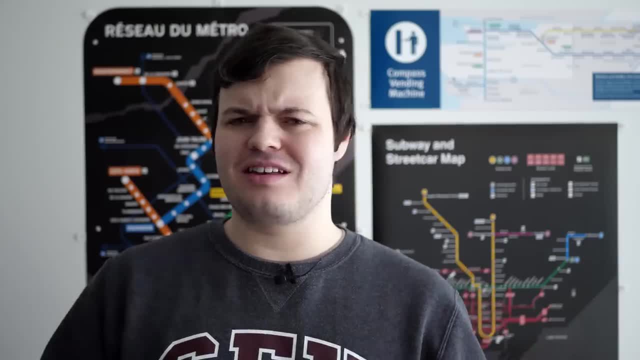 because it really helps the channel. If you are subscribed, chances are you haven't hit the bell icon, So again, consider doing so, because it really does help us keep the lights on. You're probably wondering why I'm making such a simple video, because, of course, the frequency 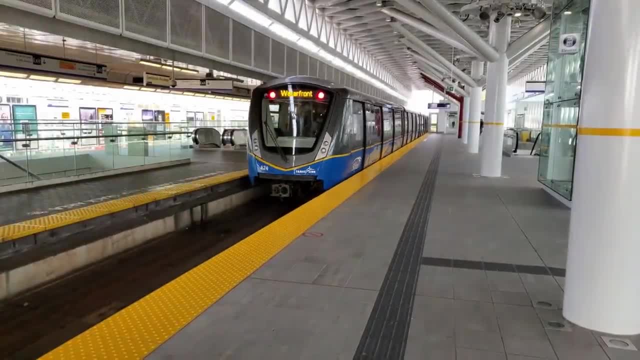 of transit. literally just how often a bus or train comes is fundamental to good transit. So if you're new here, welcome back to RM Transit. If you're new here, welcome to being good. But looking back I realized I never made a video. just about why frequency is. 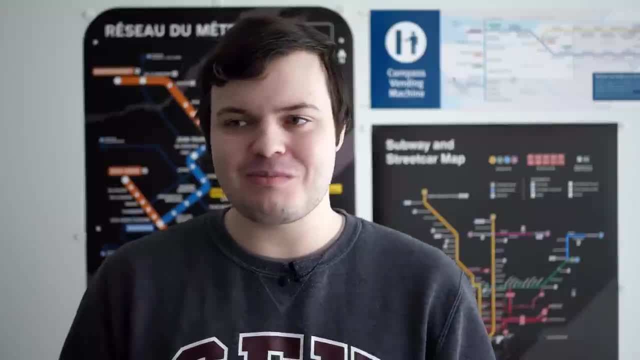 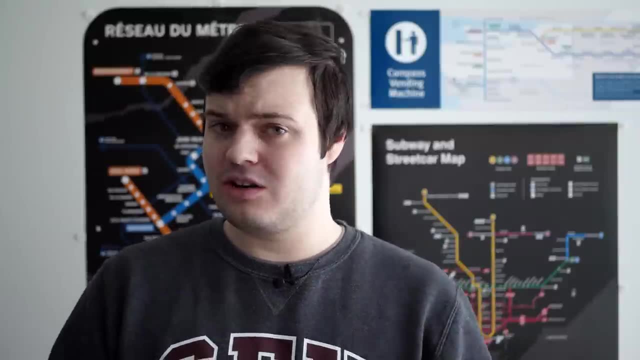 good, I've made videos on all kinds of related topics to frequency, but not the most obvious question. This sort of seems like the type of thing I should make a video about. But if you have any other basic transit stuff you think I should make a video about, let me know in the 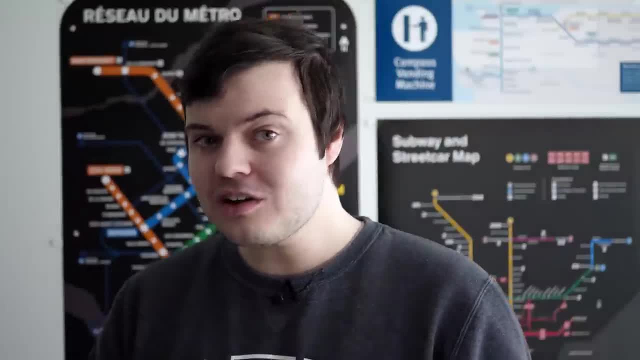 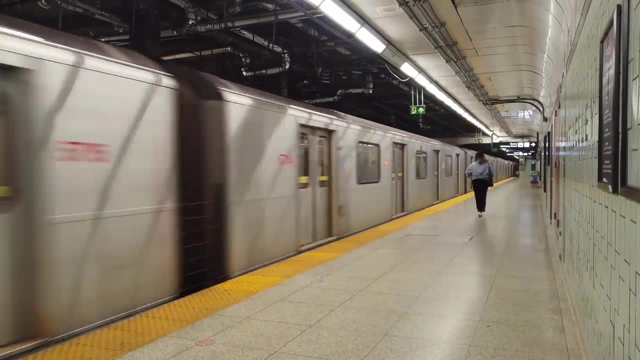 comments down below, and I'll try to make those videos as well. The first thing I'll do, as always, is bring up some examples. Something you'll notice is that most of the well-used transit out there is frequent, Though, of course, what frequent is? 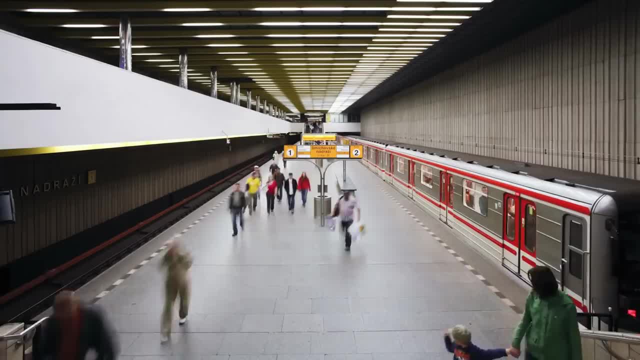 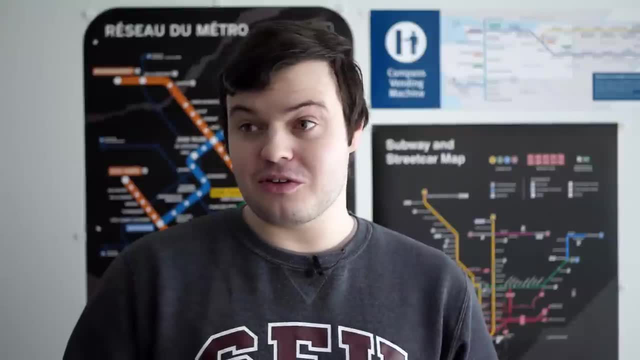 really does depend on the context. Every 10 minutes isn't really good for a subway line, but it's pretty good for an intercity train or for a bus. Now, as it turns out, the fact that these frequent services are the most used isn't by accident. 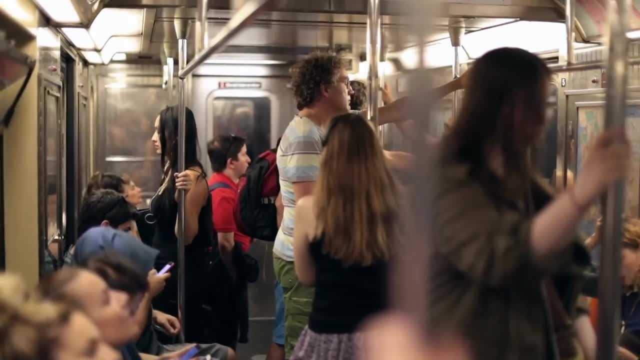 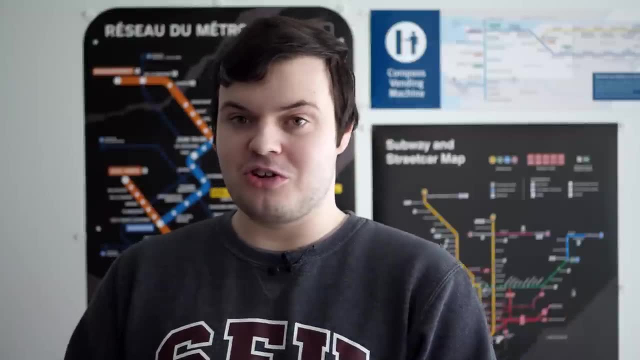 Even if transit use was really sporadic, unless there's literally no unmet travel demand, more seats is always going to give you more potential to gain riders, Even if only because transit which is not super full is incredibly comfortable to use. You see, if you run a bus, 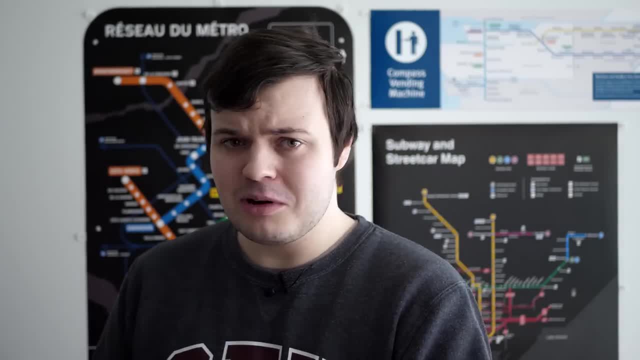 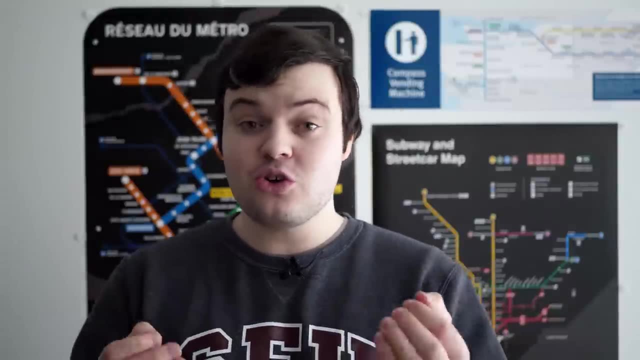 or a train line. once per hour you have a certain number of seats, But if you upgrade that to every 15 minutes you have four times as many. A train or bus every five minutes is going to triple that new number once again. Of course, frequent transit actually needs the capacity that's delivered. 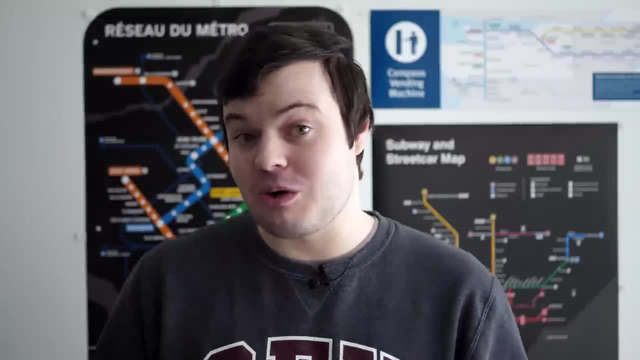 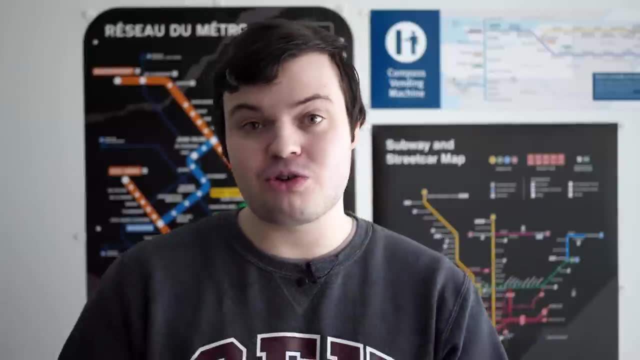 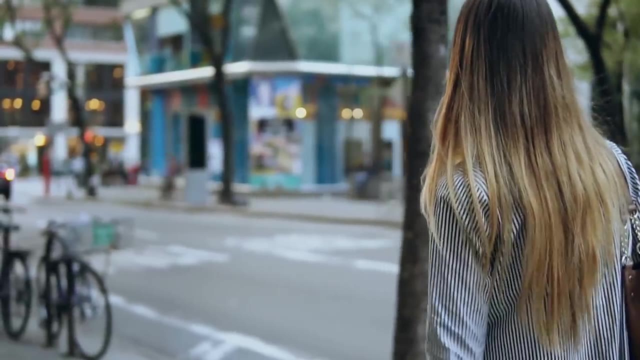 through its frequency Because, as transit planning celebrity Jared Walker puts it in his very famous book Human Transit, frequency is freedom, And this is the most salient description of why frequency is good that I think exists out there, At least on the basic level. Frequent transit lets you travel whenever you want to travel. 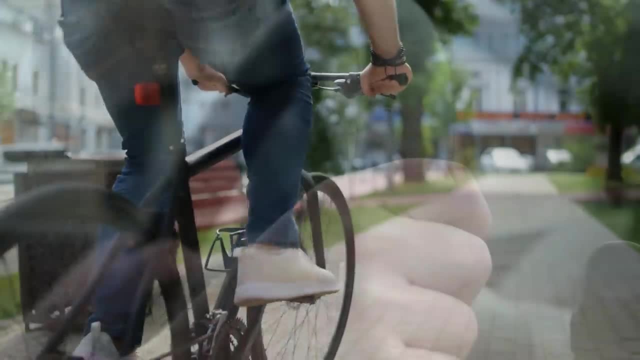 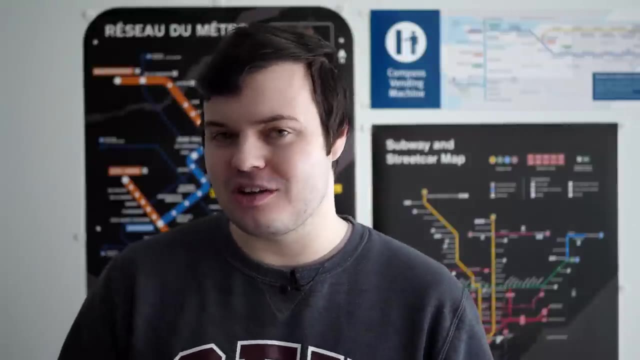 which all compelling modes of transportation- be it walking, cycling or, yes, even driving a car- all allow you to do. Now, car analogies will always be somewhat controversial in the transit space, but around the world, cars are one of the main things competing with transit, And so I think 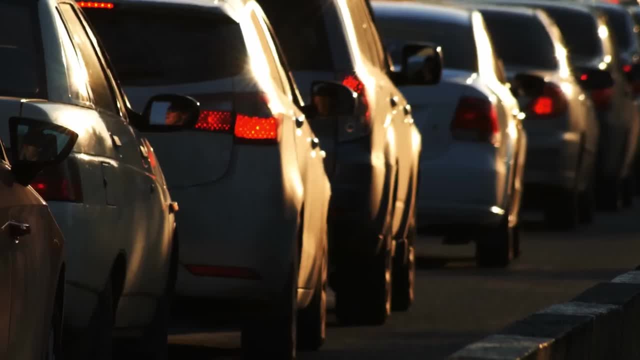 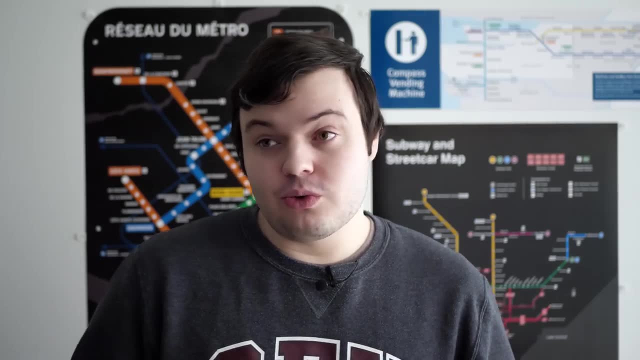 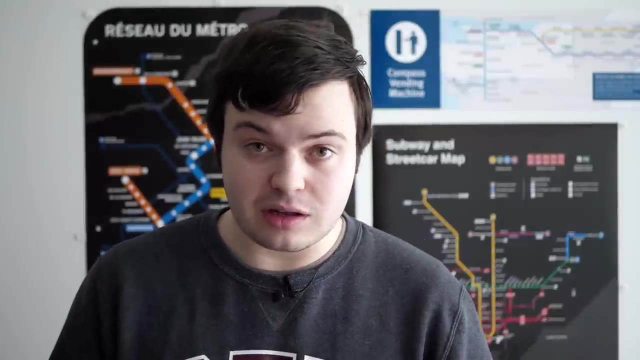 it's worth doing some comparisons to at least see what we can learn from what makes cars popular Now as much as transit. people like me do sometimes push back on this. it is absolutely true that being able to get into a car and go wherever you want whenever you want is a hugely powerful thing, even if just psychologically. 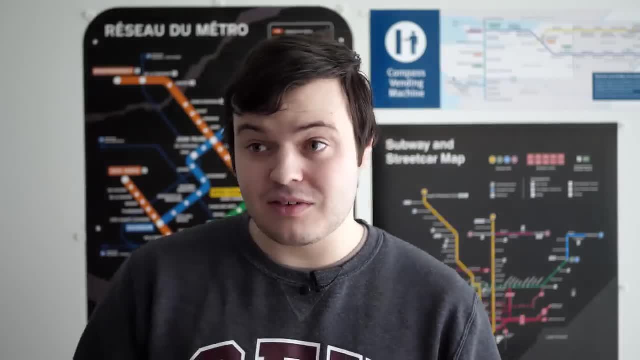 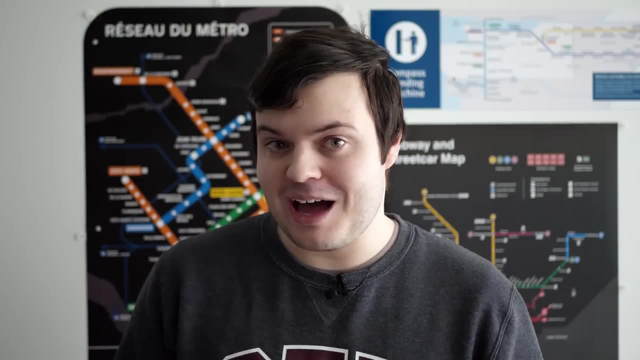 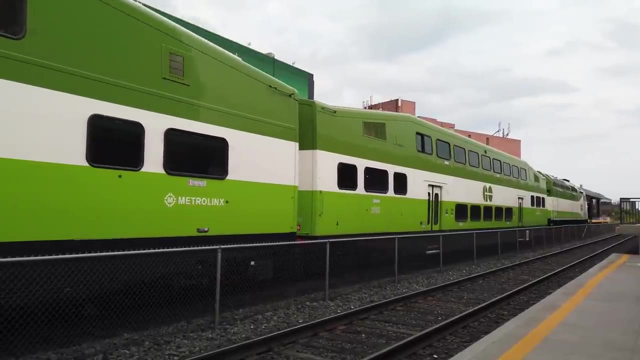 Cars have tons of negative aspects that transit doesn't have, but just the benefit of feeling like I can go whenever I choose, even if it's at 3am, is really impactful. Now, as I sort of alluded to before, lower frequencies on transit can sort of be accepted on longer trips, And the reason for 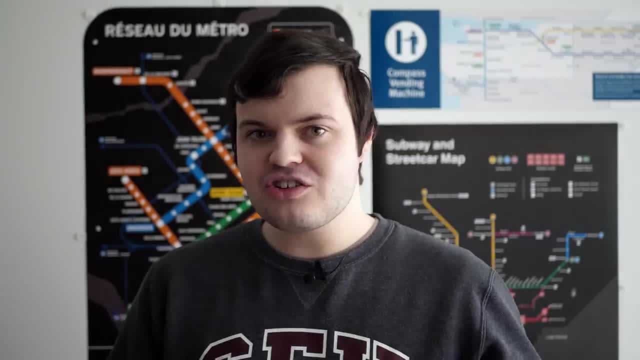 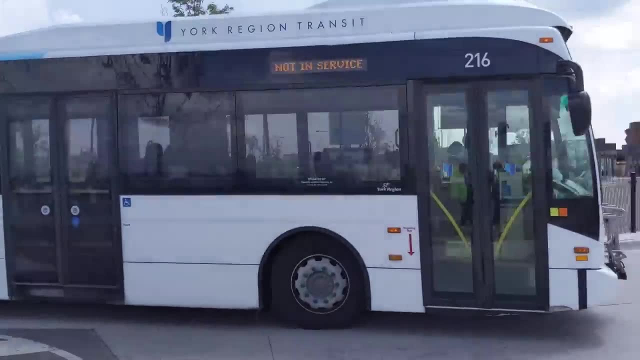 this can be explained through this video, which I'm going to show you in just a moment. So imagine taking a short trip from your home to like a suburban shopping mall or something like that, on a bus that runs really infrequently, let's say every hour, which is sadly all too common in 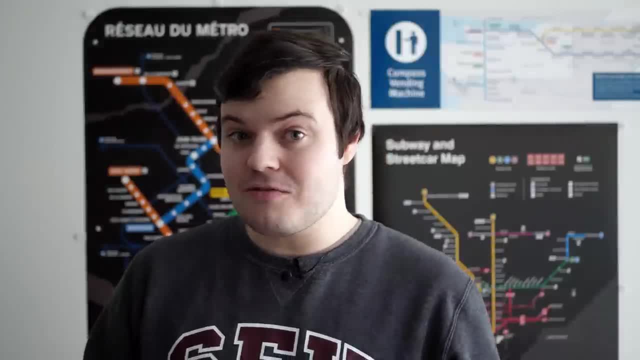 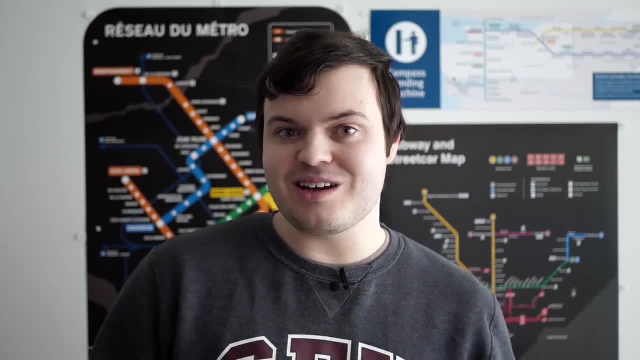 North America. Given that buses, even those with dedicated lanes, often have lower average speeds than cars because they do have to make stops for people to get on and off, It's going to be basically impossible for that hourly bus to compete on travel time alone with a car. In fact, it's a really good idea to take a bus to a mall and back in the time. you might end up waiting for that bus, And I think people are well aware of that when they see an hourly bus service. Of course, driving may still well be faster, even if the buses run every 10 or 15 minutes. 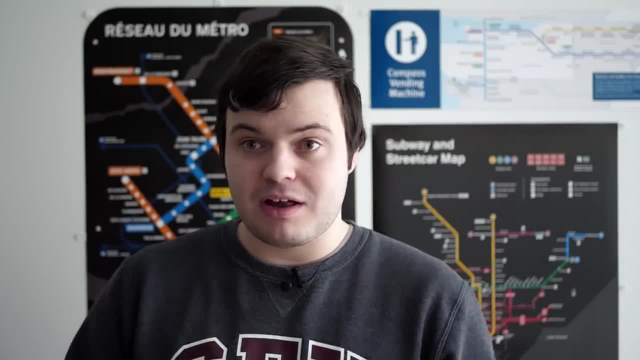 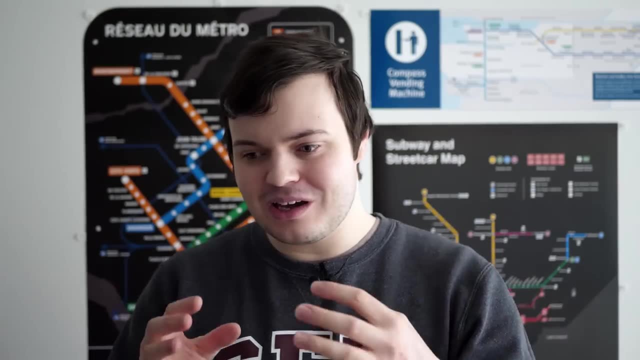 but the gap is a lot smaller And that's where the benefits of a bus that a car just cannot compete with- like being able to take a nap or go on your phone or just not focus on doing an active task the entire time- really starts to compete with the allure of actually driving. 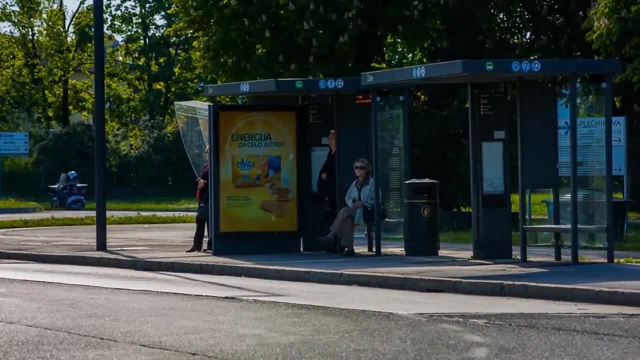 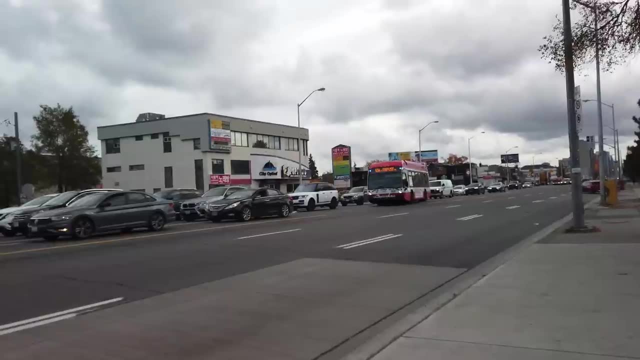 There's also a lot of other benefits that you might find that a bus can't compete with, Like a very powerful psychological effect of just sitting at a station or transit stop while other vehicles drive by you. Time spent sitting still just feels unproductive, more so than even riding. 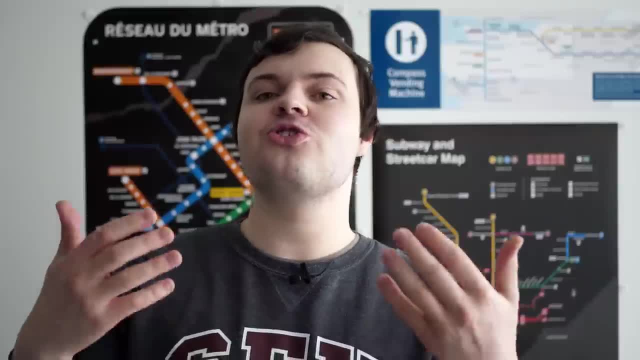 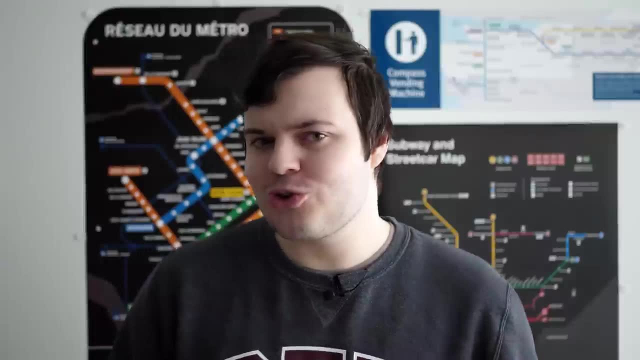 on a vehicle that's going really slowly, because then at least you're still making progress. Of course, making longer trips in a city with infrequent transit gets even more painful. Of course, transit networks based around transfers are way more useful generally than 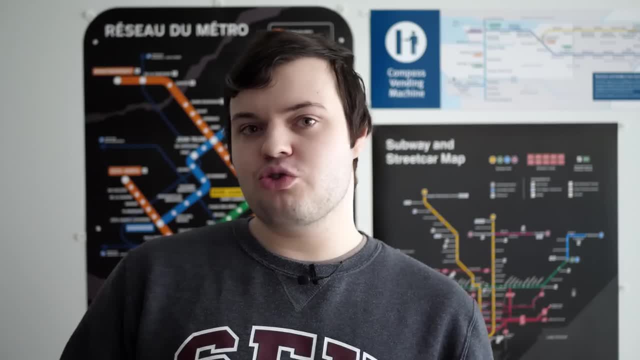 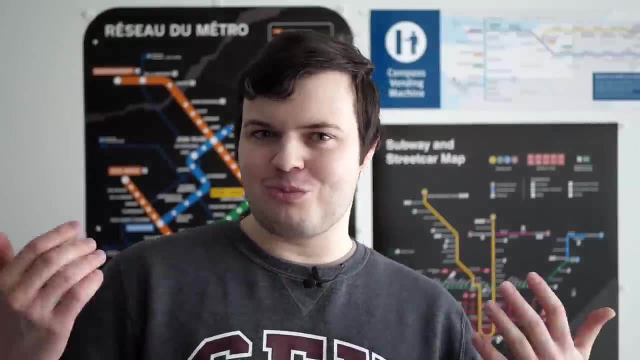 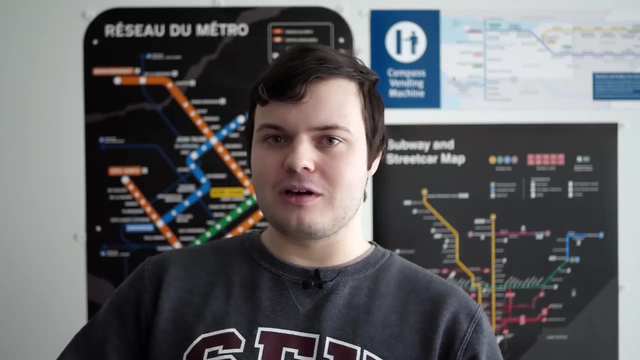 transit networks that are based on a lot of one seat rides because you can transfer from one line to another to go almost anywhere relatively quickly. That said, transfer based networks actually become worse than one seat ride based networks once you start having really poor frequencies, because the only thing worse than waiting for your bus for maybe 30 or 40 minutes 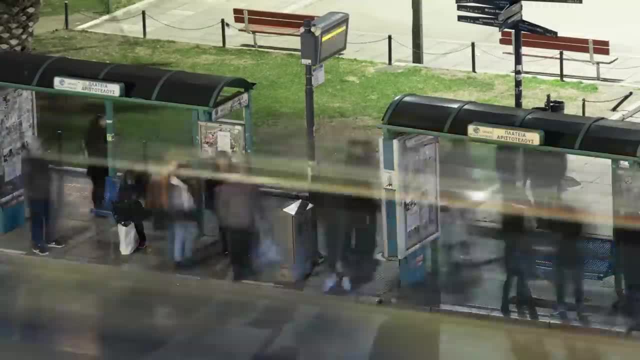 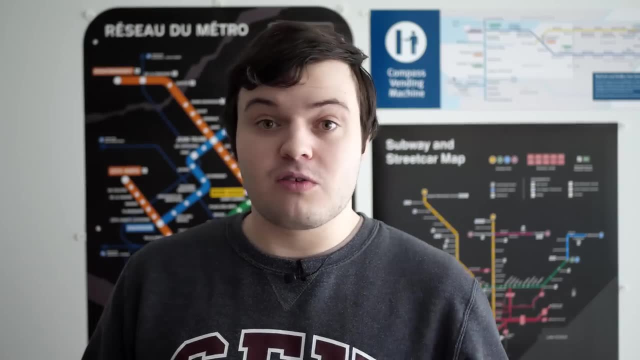 is having to do so twice. This punishes people who use transit and make sure that nobody privileged enough to have another option will actually use it, And I think honestly that's a large part of what causes transit to be stigmatized in certain places. There's a positive side to this as well. 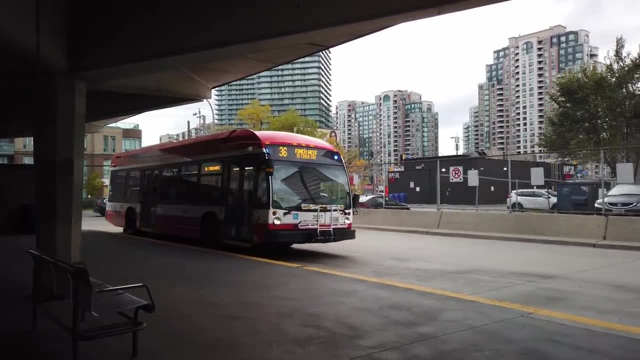 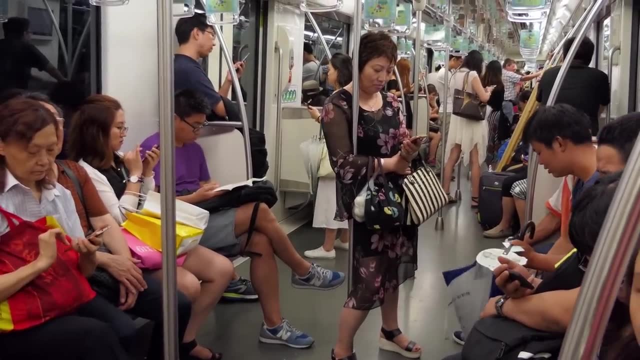 though, As you can see, with system after system that has increased their service, ridership tends to follow very closely, Because once transit becomes competitive and convenient, taken as a whole, it becomes way more popular. Cars are never going to be able to compete on things like price. 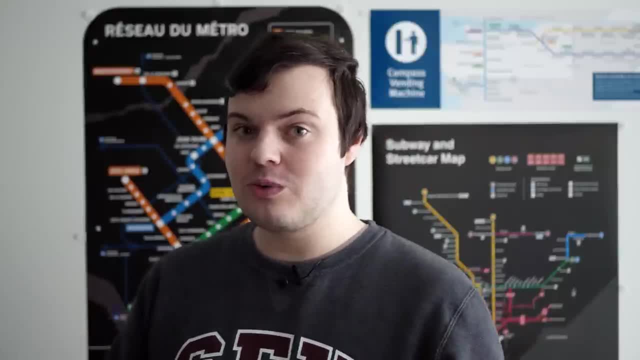 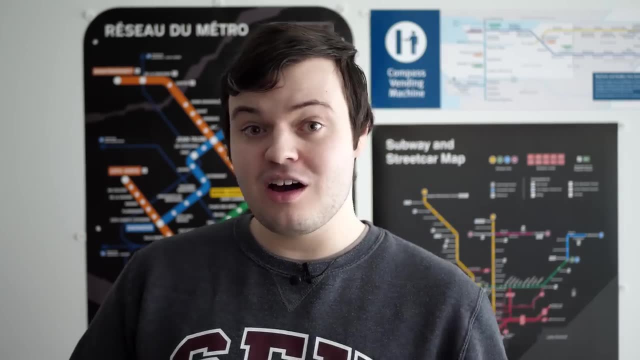 At the same time, you're probably going to need the capacity that frequency delivers, because, unlike with just having bigger vehicles, like, let's say, a double decker bus or a train, that's just twice as long. when you add frequency, you actually improve the. 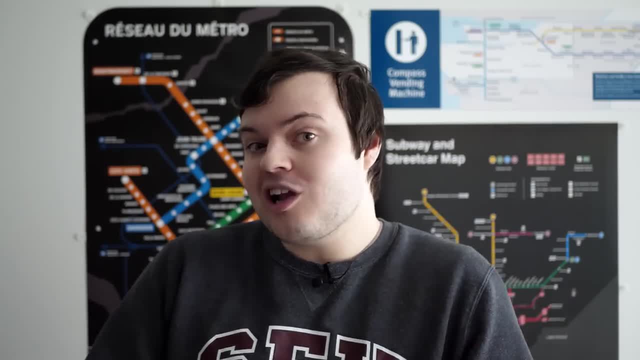 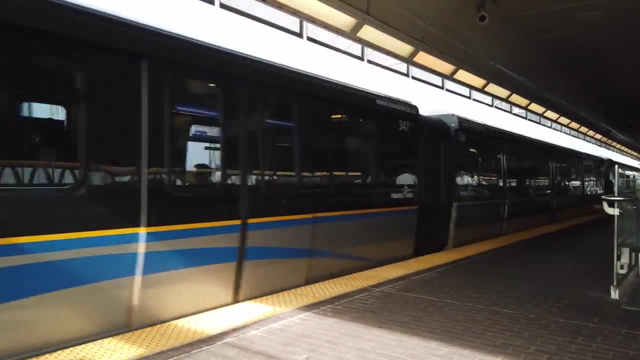 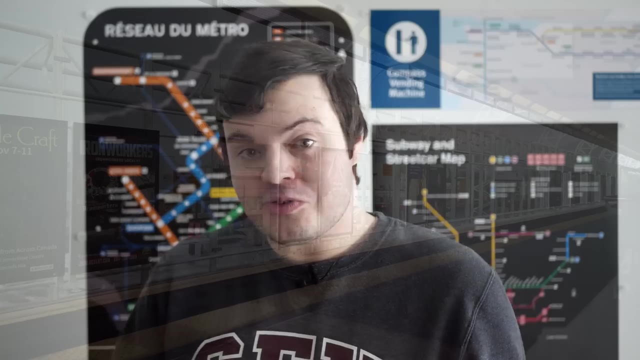 level of service of transit, which means you make the quality of transit better. That's why it's really important to focus on building capacity through frequency. first, because you get all of those upfront benefits of making transit better that you wouldn't get with just having a bigger train that still comes in frequently And, of course, much like the pain of 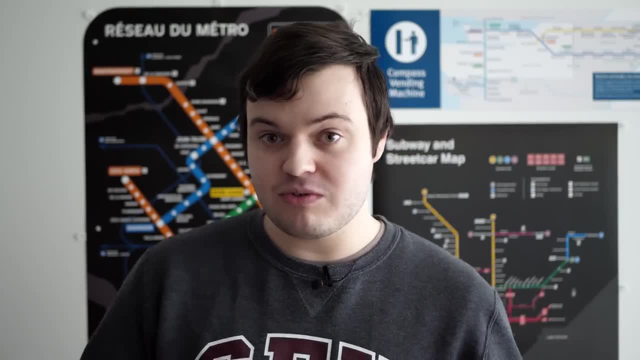 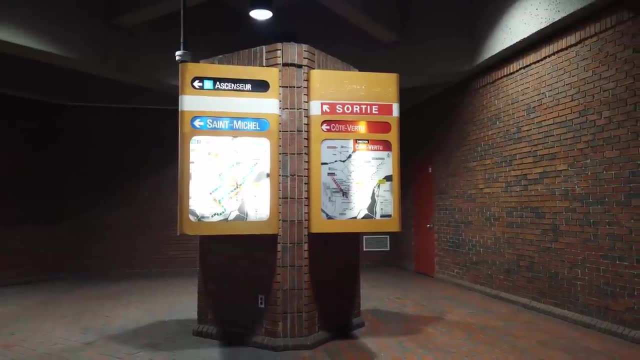 transferring is amplified, the number of times you have to transfer, the benefits of really frequent transit are amplified over trips that have more and more transfers, since you can conveniently transfer when needed. Your next vehicle is only a few minutes away. The TLDR of this is that nobody wants. 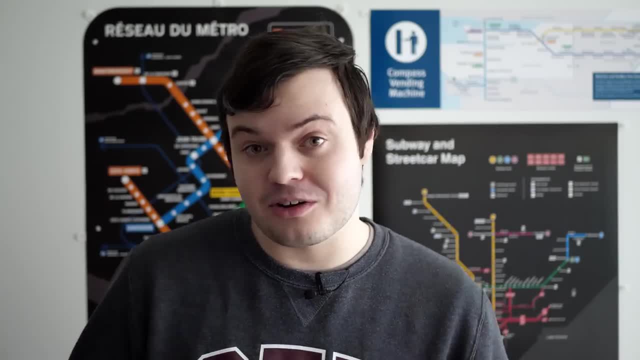 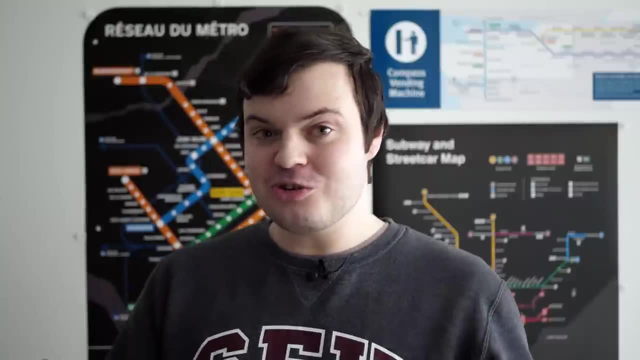 inconvenient or infrequent transit. These things do come together And when you don't have those things, transit tends to become popular and you need more capacity Because, honestly, as long as your transit runs, often it's going to start being pretty competitive with driving. 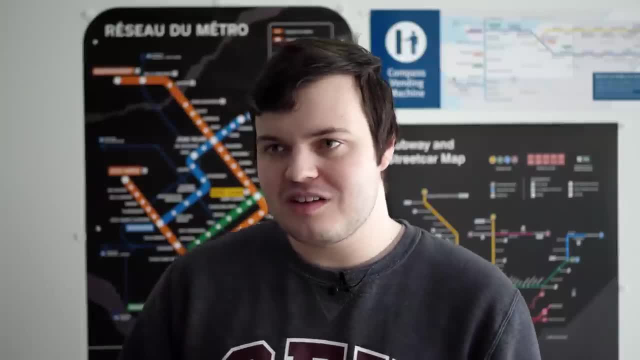 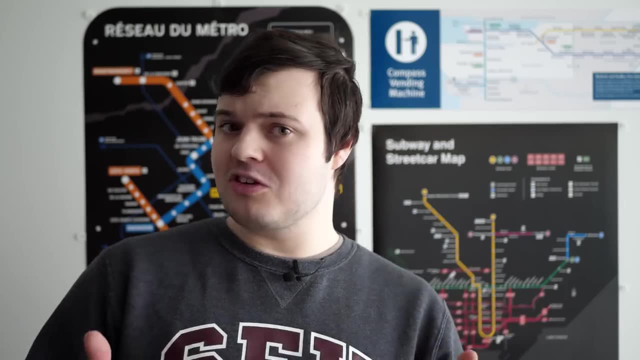 even if it's slower. Now, one of the deceptive things about frequency is, as I mentioned before, it reduces your need for gigantic vehicles, And this can really distort the dynamics around what people think is appropriate, And that's why it's so important to have a transit system that's 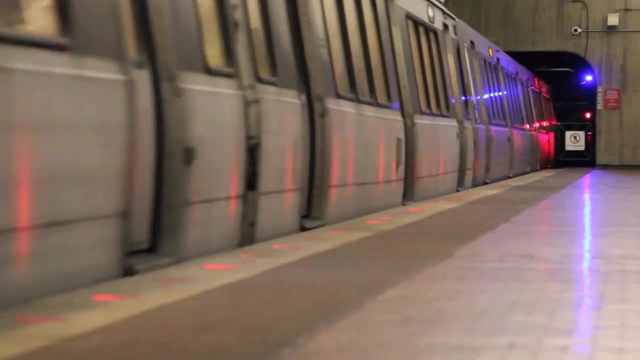 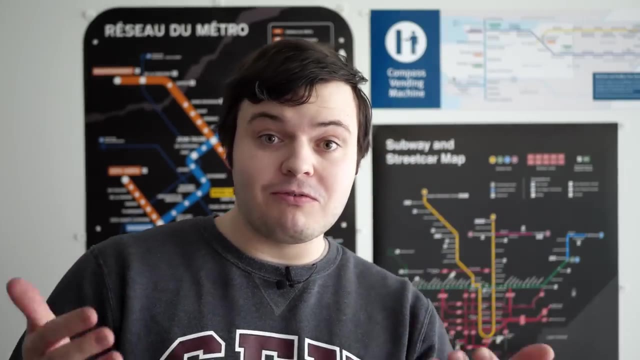 appropriate. In the United States, a lot of subway systems have trains that are 120 meters long or longer, And, yes, I'm going to use metric, Come on, But these trains tend to run fairly infrequently And what's interesting is that the ridership you see on these lines tends to be similar to 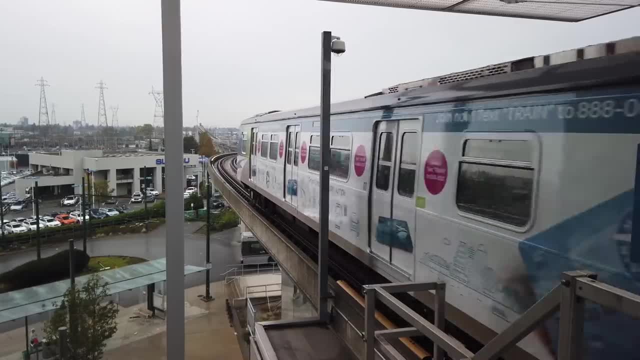 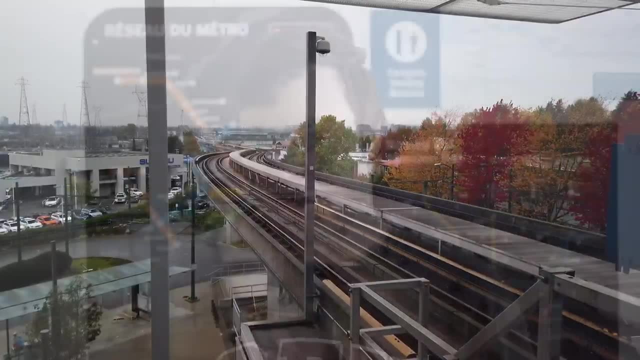 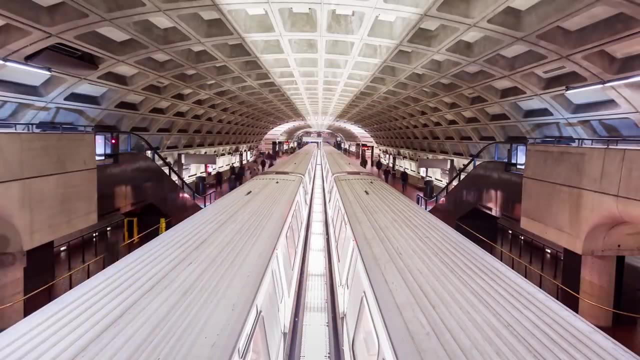 what you see on smaller lines in places like Vancouver or Madrid, And so it can be tempting- and I have fallen into this trap before- to suggest that you could simply build Canada Line style mini metros in places like Washington DC, which would satiate all the demand. The issue with this is that it doesn't account for the 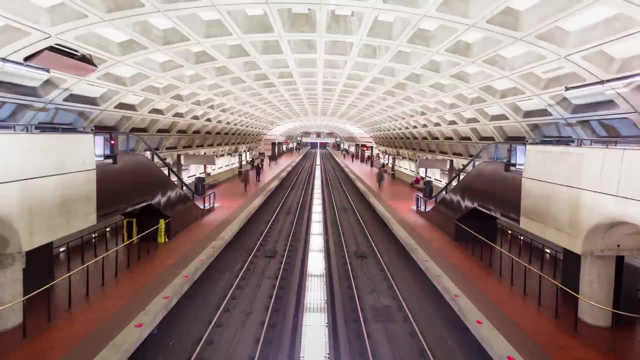 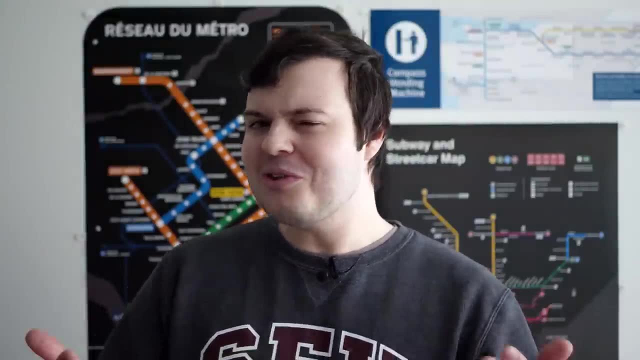 massive ridership uplift you're going to see when you start running trains way more frequently. Now, that's not to say you couldn't make trains in a lot of American cities a lot smaller and be totally fine, But there's a reason why cities like London and Paris still tend to use trains around. 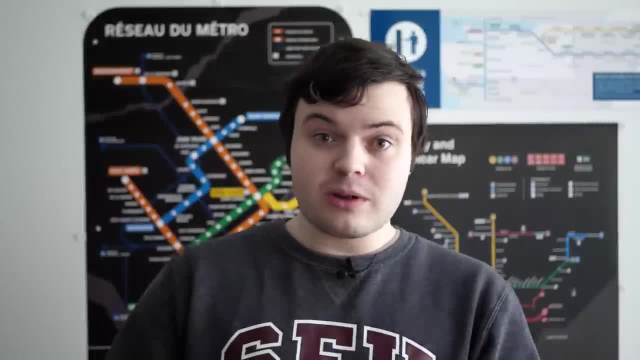 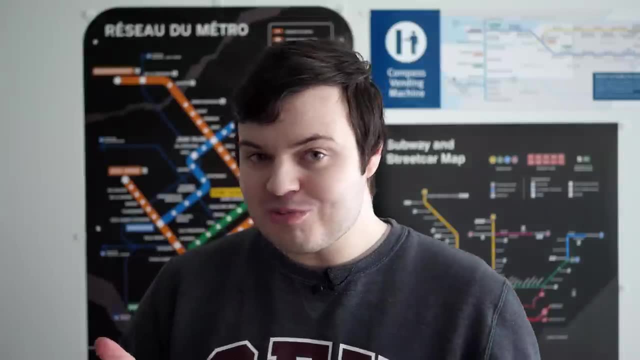 100 meters long, especially on newer lines. Of course, if you're building above ground, this matters even less, because your prices are less impacted by having larger or smaller trains. Now there's probably a PhD to be done somewhere talking about where the limit of more frequent transit becoming more popular is. 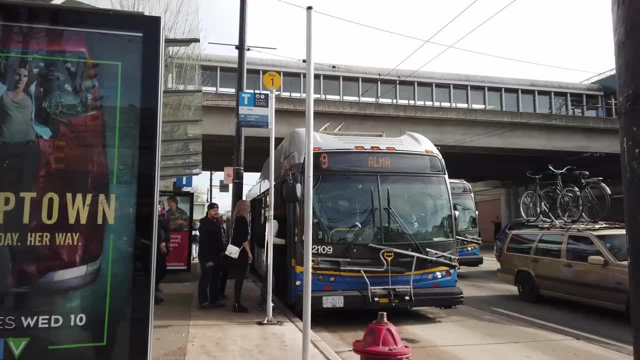 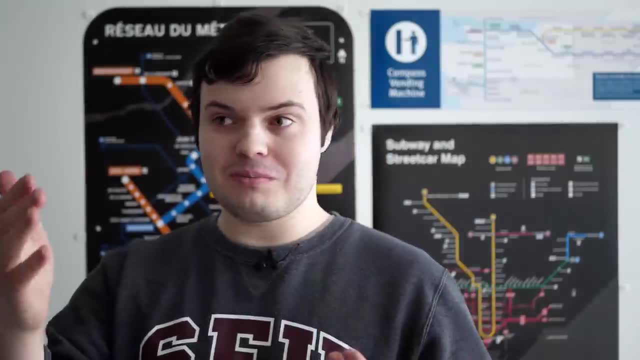 but we don't really know, as far as I can tell. We know that there's a floor where people will accept transit as frequent of about every 10 to 15 minutes, but it's not clear just how frequent becomes frequent enough When you talk to people in cities where trains run every 90 or 100 seconds. 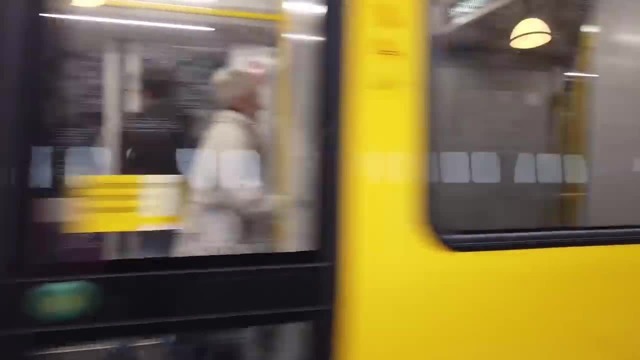 on metro lines. they tend to be really happy that they can just wait if the train is crowded and get on the next one. Of course, there have long been a lot of people who want to get on the next train, but they don't know how to get on the next train. 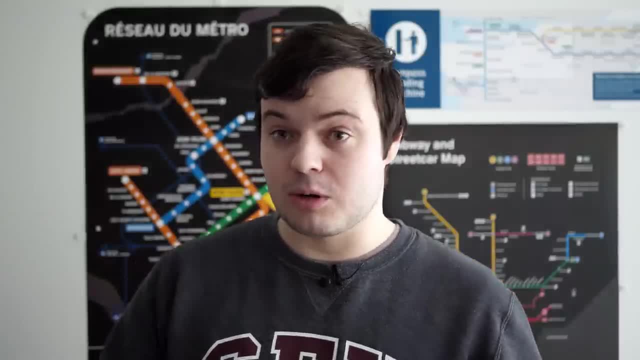 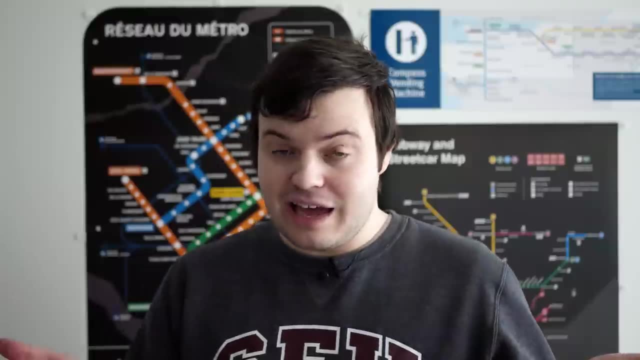 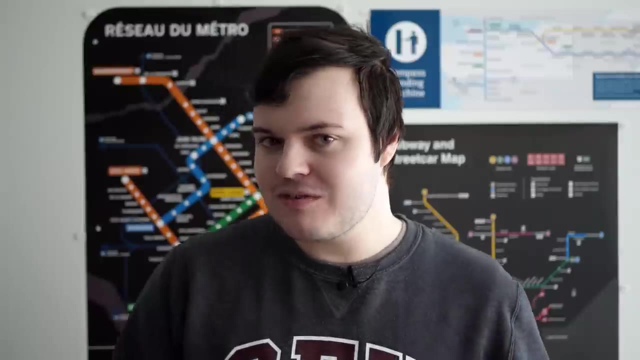 Not only because of one of the commonly stated factors, which is labor, but also because we didn't really know how to design stuff in the optimal way to make frequency possible. We actually have historically had systems that operate super frequently on things like older subways and streetcar networks. Where we've really innovated is being able to make them much faster.